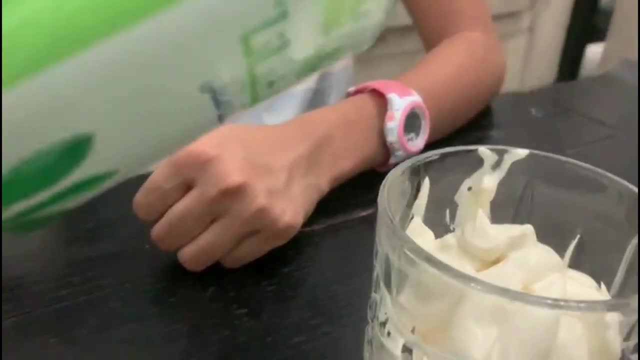 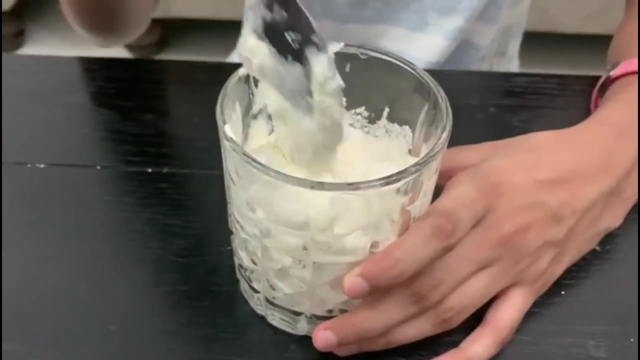 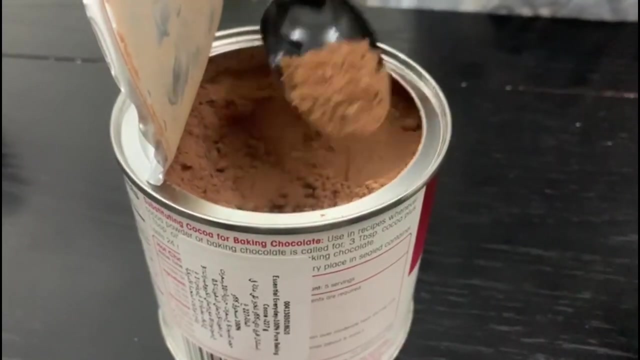 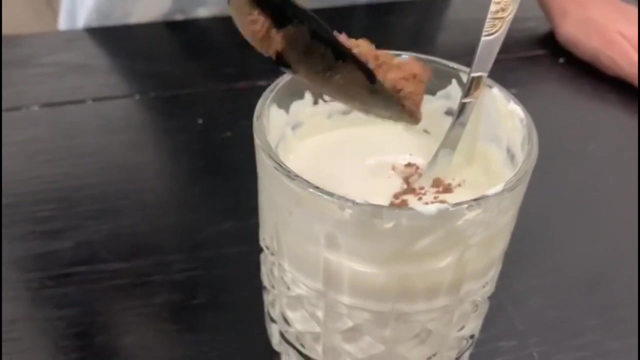 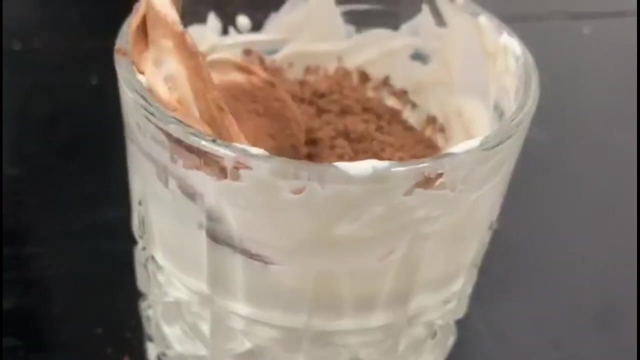 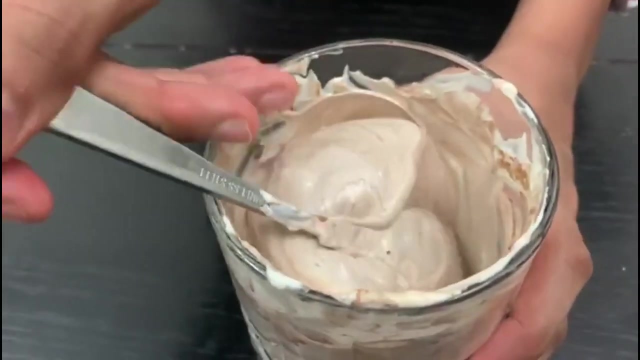 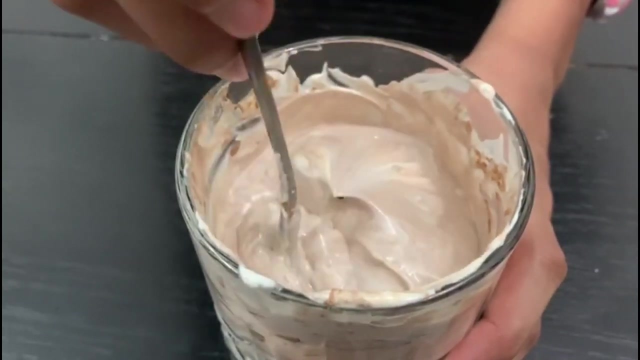 sugar. And now I'm going to be mixing this, and you can add as much sugar you want, as per your taste. Now I'm going to be adding half a teaspoon of cocoa powder. You can do it as per your taste. Pour this gently, like this, until all the thick cream turns into this light brown color. 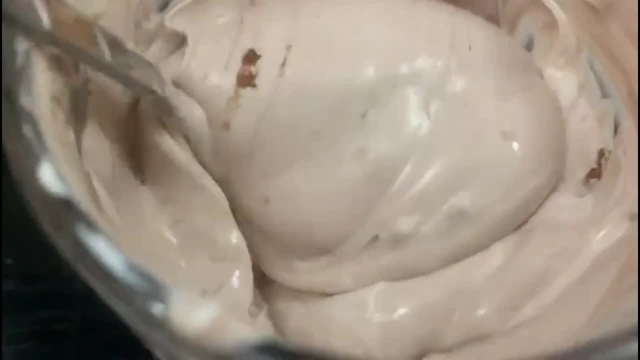 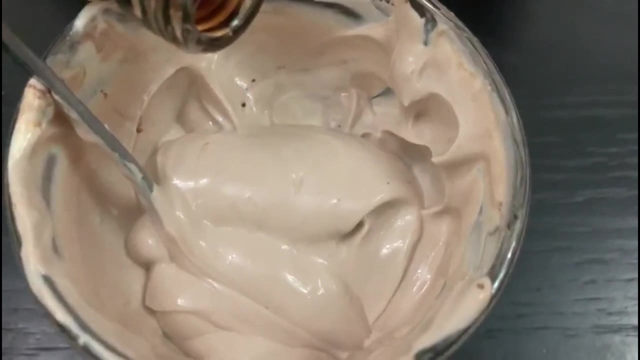 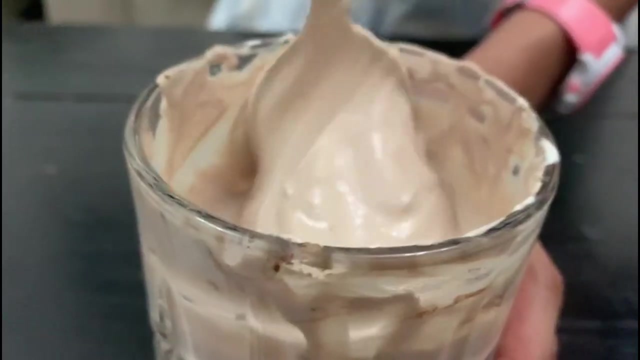 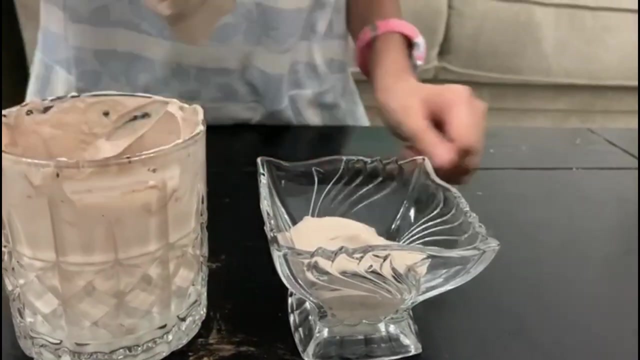 Now you want to put a few drops of vanilla essence, and very few. This part is also optional. You can do it if you want. The vanilla essence is smelling amazing. It smells like really tasty. Now I'm putting this mixture into the serving bowl. 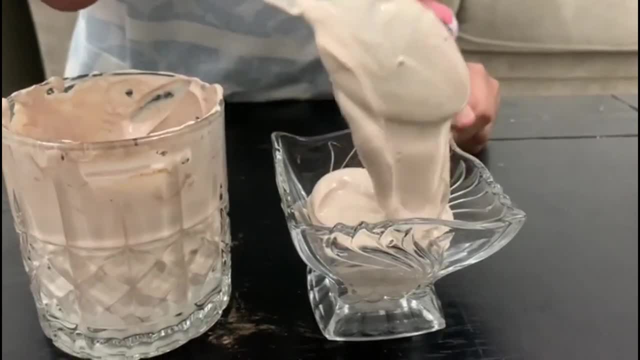 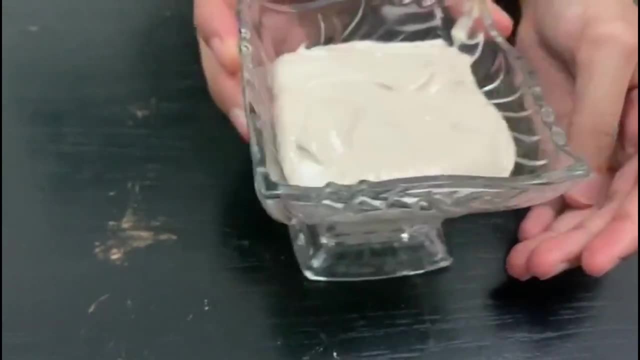 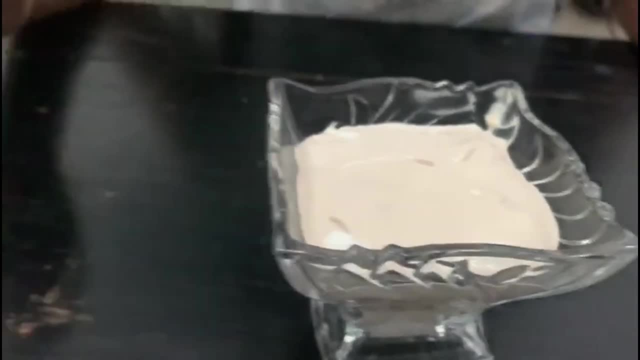 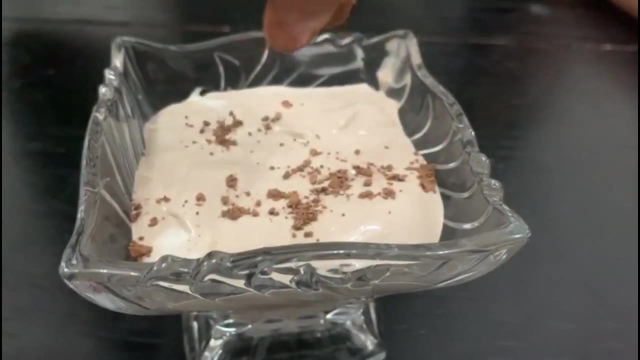 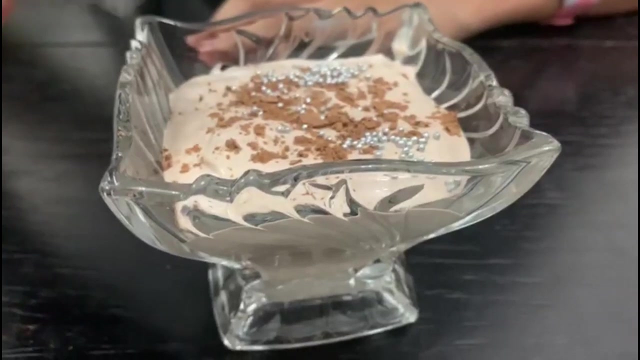 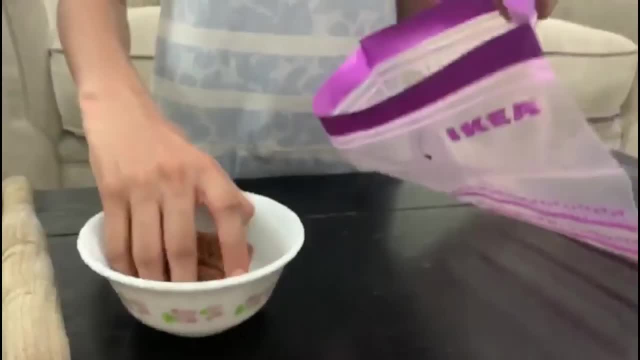 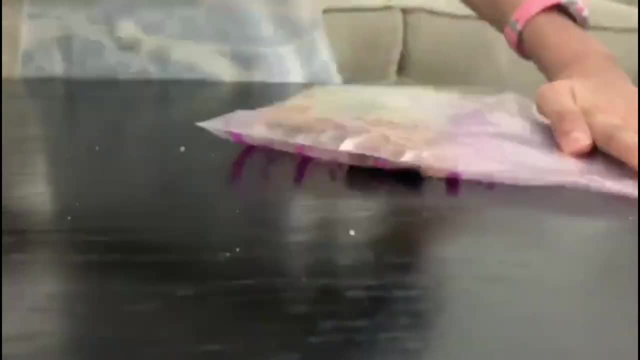 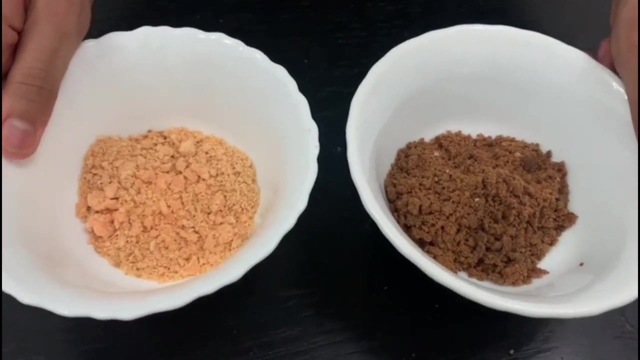 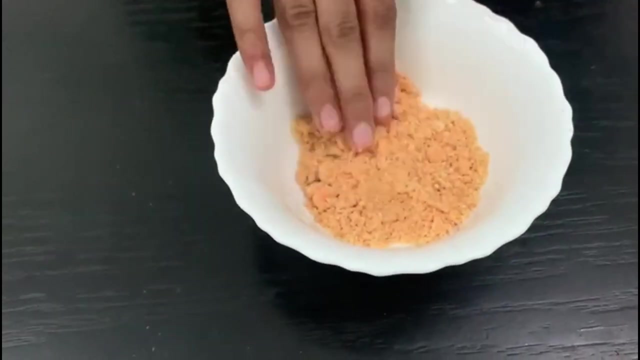 Now I'm going to be adding these silver balls as a topping. It's also optional, so you can do it if you would like. another ziplock bag so I can grind the bourbon biscuit. now we have almost fine powder. see, yeah, now I'm going to press this down, just flatten it. 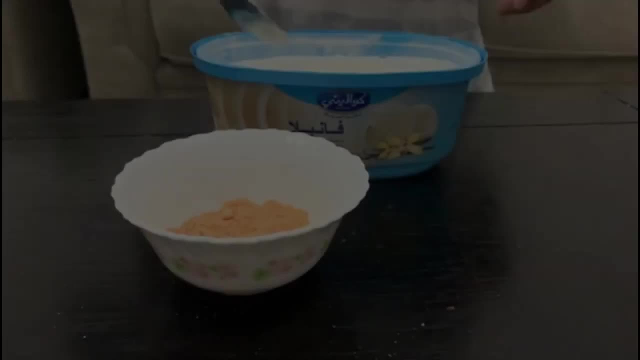 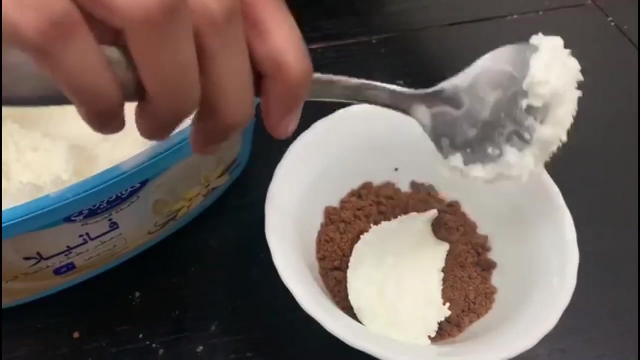 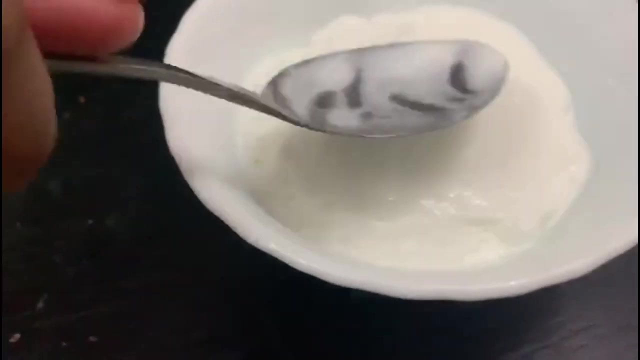 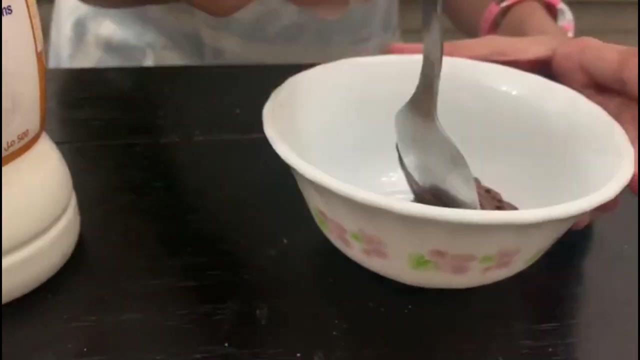 it. now I'm going to be pouring in the ice cream. you can put as much as you would like. now we are going to just flatten it out, so to be nice and level. so, guys, now I'm going to be preparing the Nutella dessert, since Nutella is really thick and won't make a good grizzling. 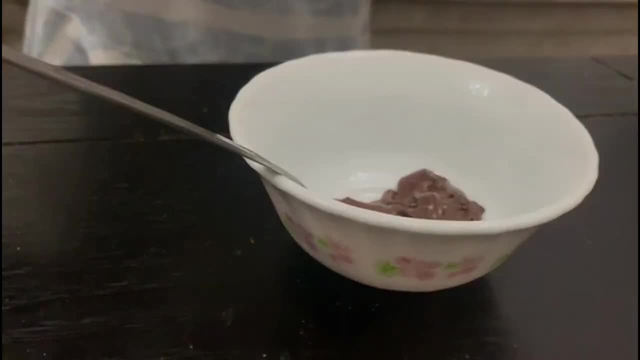 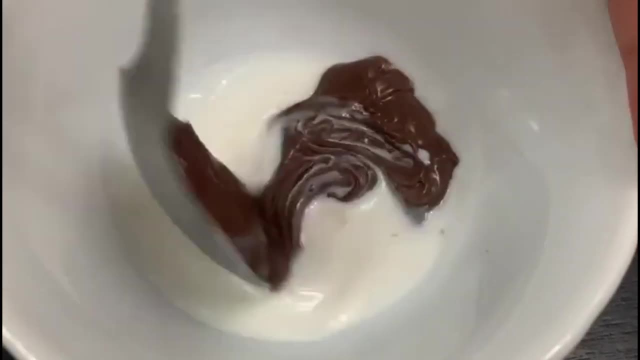 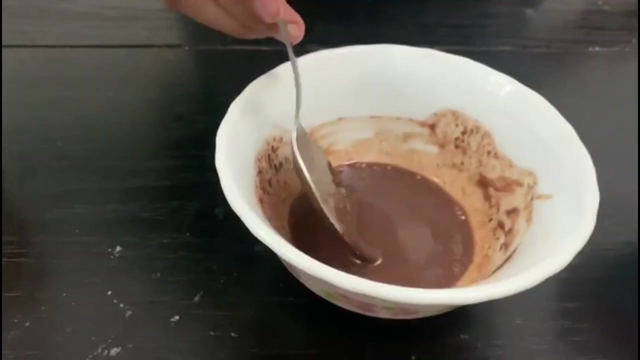 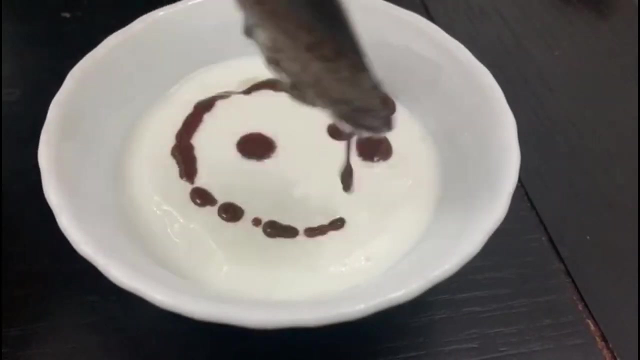 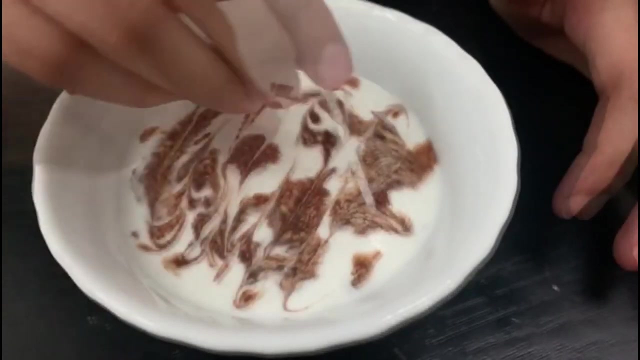 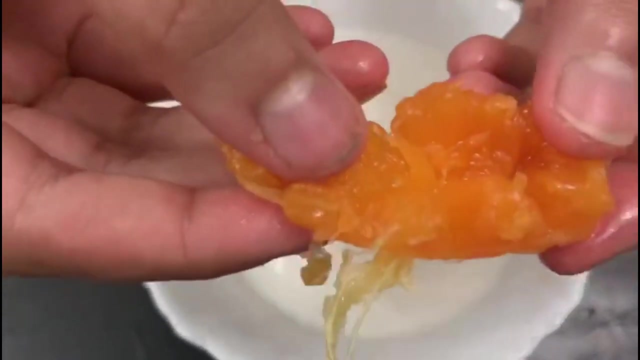 shape. I'm going to add a little bit of milk. the mixture is ready. I'm going to be drizzling it like this. I'm going to use a toothpick to cause this type of a design. this one is the orange biscuit. I'm going to be adding cubes of orange. 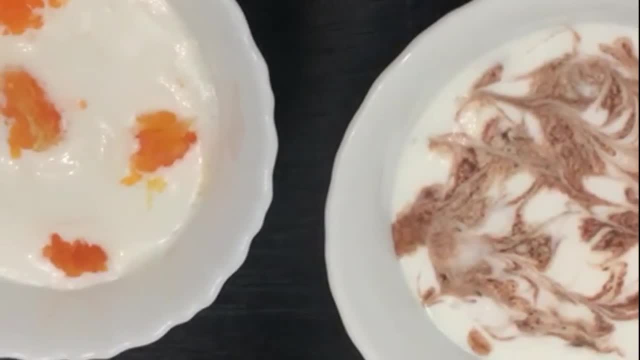 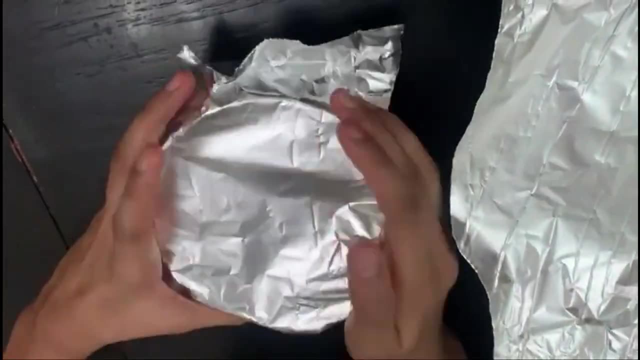 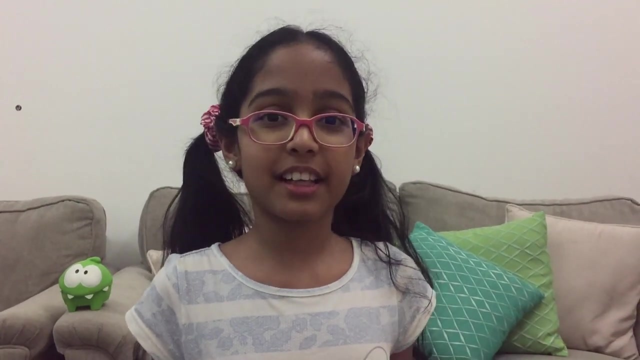 now, it's almost done. you just need to put it in the freezer. before that, we need to cover it with foil, so so, so, so. so the last and the last and the last and the third recipe is powder. the third recipe is powder. these are the ingredients you are going to be needing. 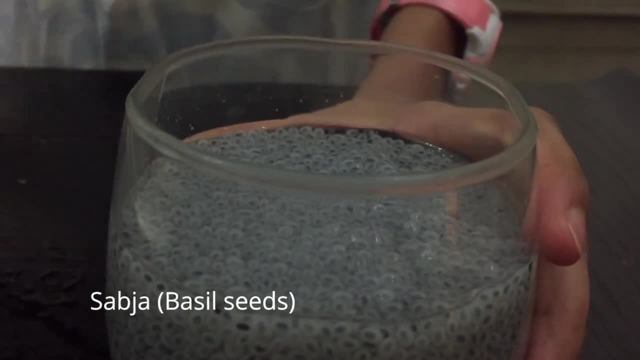 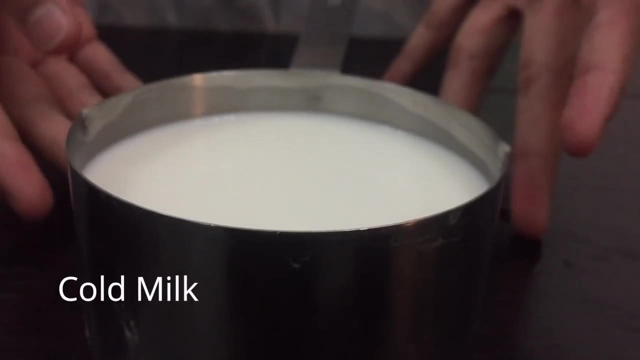 these are the ingredients you are going to be needing. first is sabza. you have to keep it in water for at least 30 minutes. next ingredient is milk. next ingredient is milk. I've added sugar to it to make it a little sweeter and ensure it is cold milk. 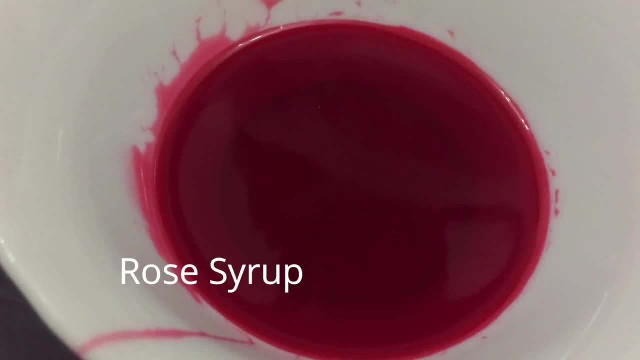 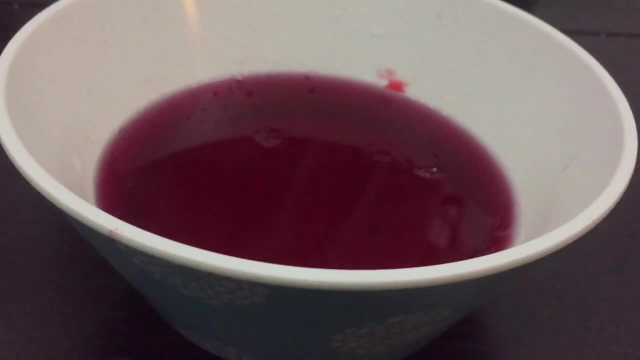 and ensure it is cold milk. here we have rose syrup. here we have rose syrup. here we have is jelly. here we have is jelly. you can make it at home. it's really easy to make and you can also find it ready made at the store. now we are using vanilla ice cream. 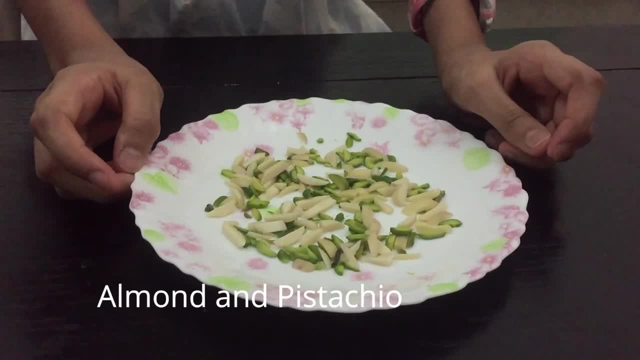 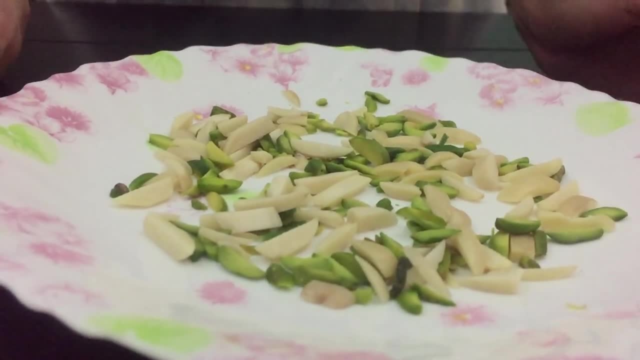 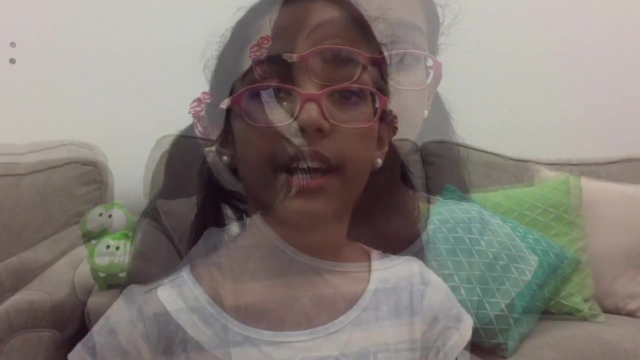 here we have awesome nuts, and I have not chopped this at all, I just found it ready made at the store, because I actually promised you guys in the beginning of the video that I will not do any shopping if you don't have any chopped nuts or you. 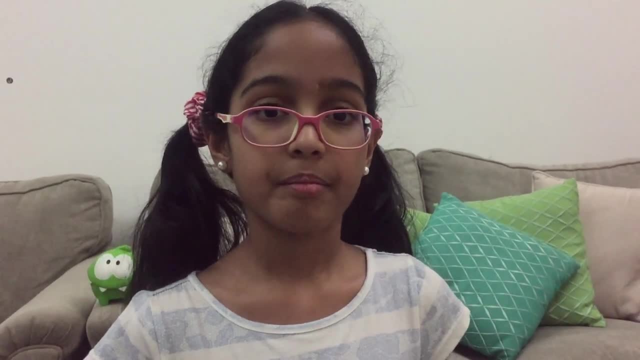 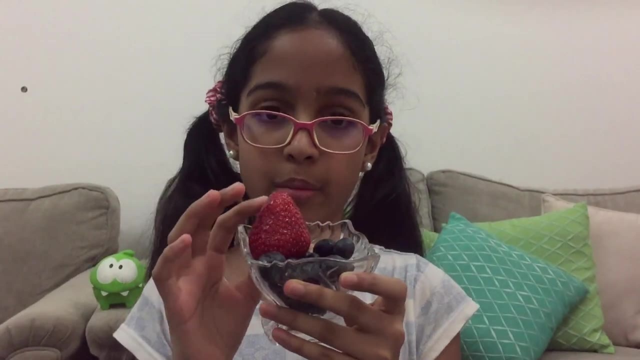 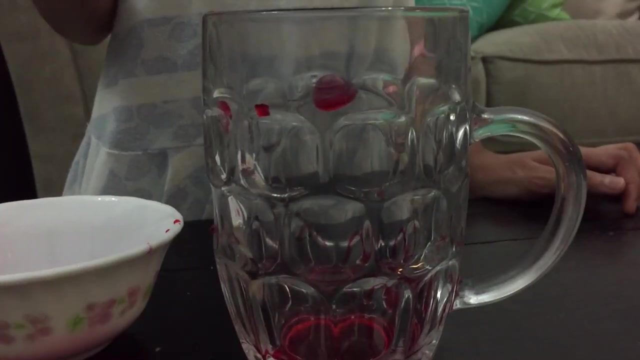 can't find them in the stores, then you can just grind them. now. my other topping choice is blueberries and a huge strawberry, and where we're going to be making the falooda is this huge mug. now I'm being going to add the rose syrup. 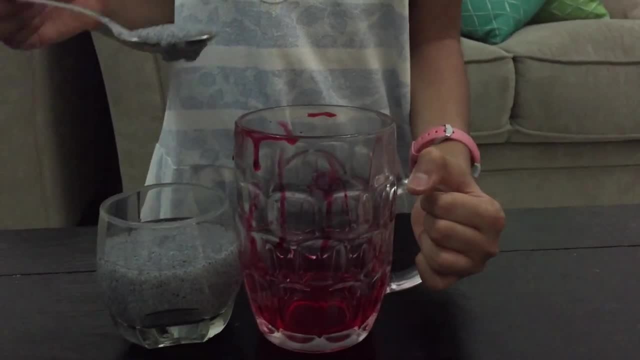 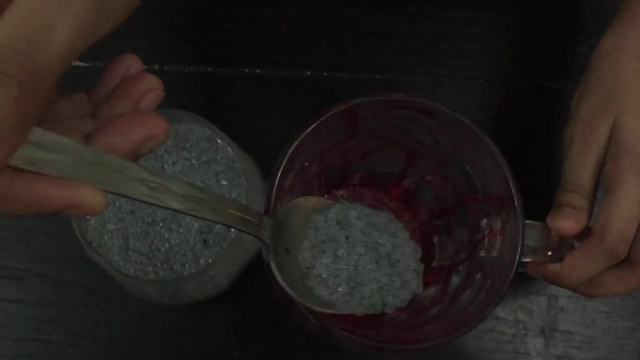 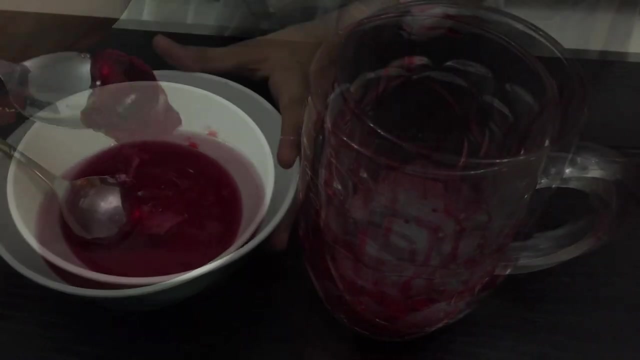 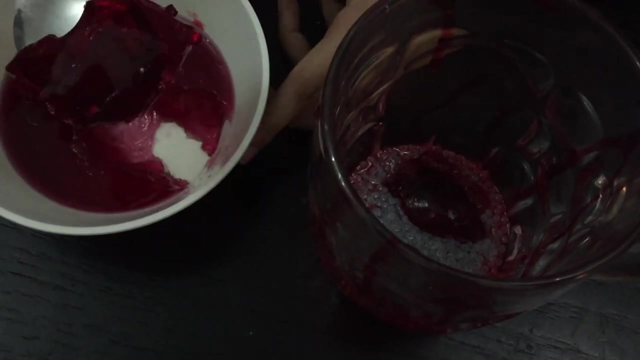 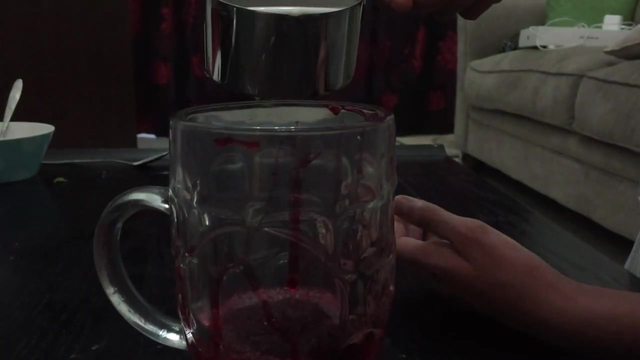 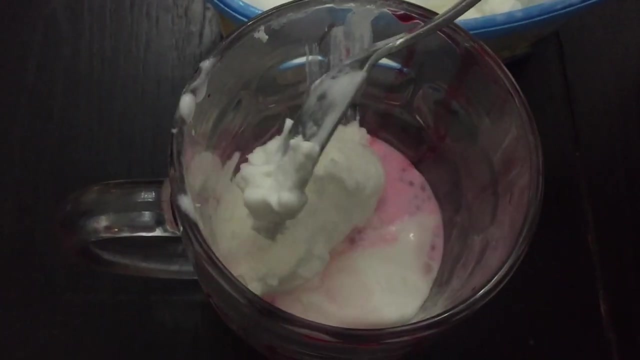 now, I am adding the sabza into this mug. I am adding the jelly now. now, I am going to be pouring a little. now I am going to be pouring a little milk, milk. I am adding a few scoops of ice cream. I am adding a few scoops of ice cream. 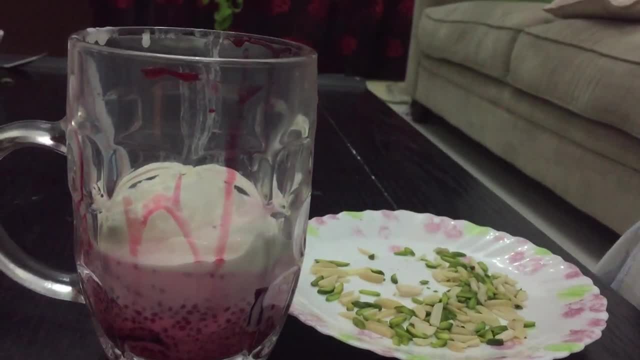 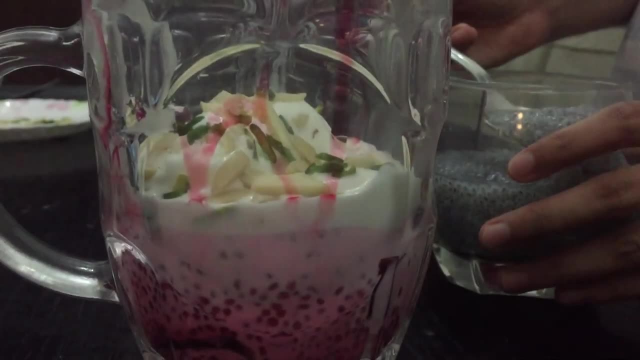 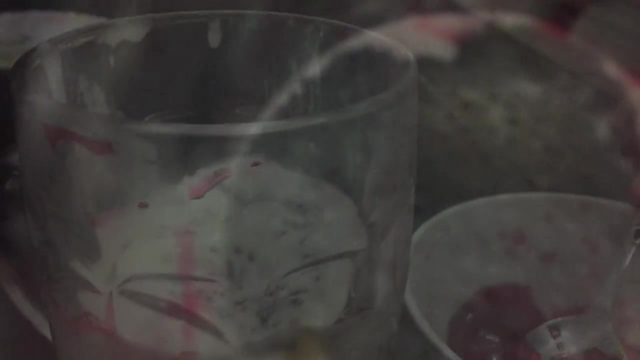 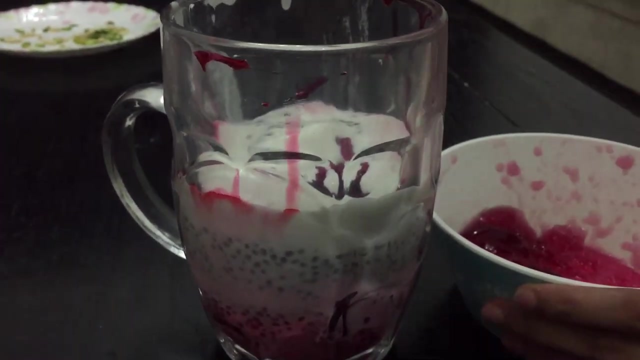 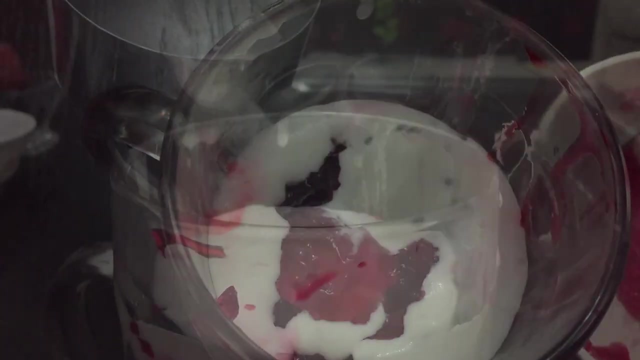 now I'm going to be adding chopped nuts. now I'm going to be adding chopped nuts. I am again putting a layer of sabza. now you're adding the jelly on top again. now you're adding the jelly on top again. Now we are adding the milk. 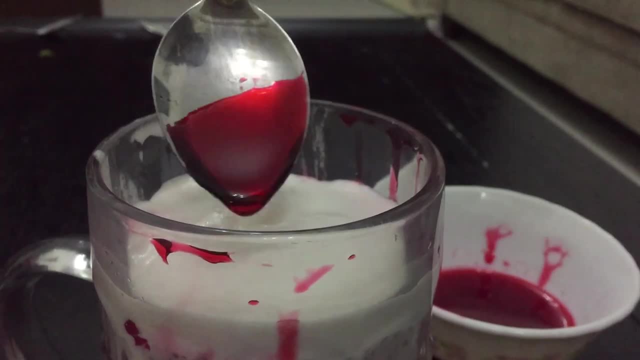 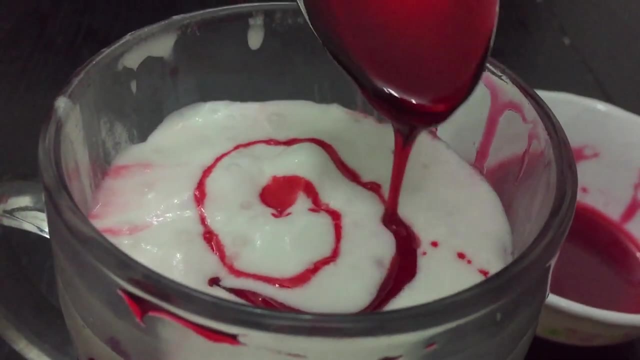 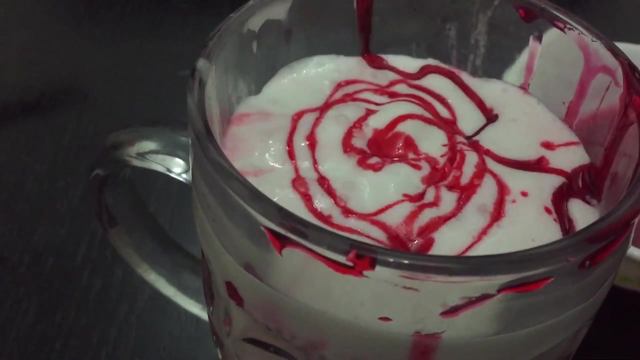 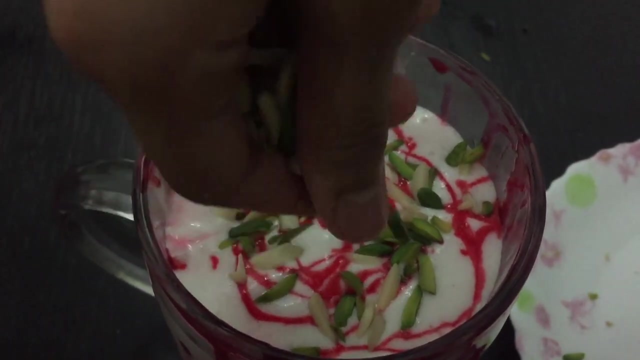 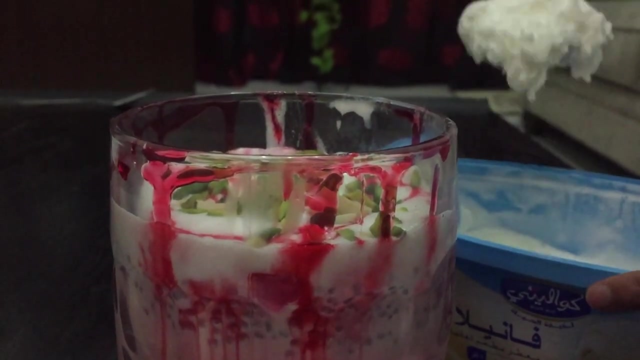 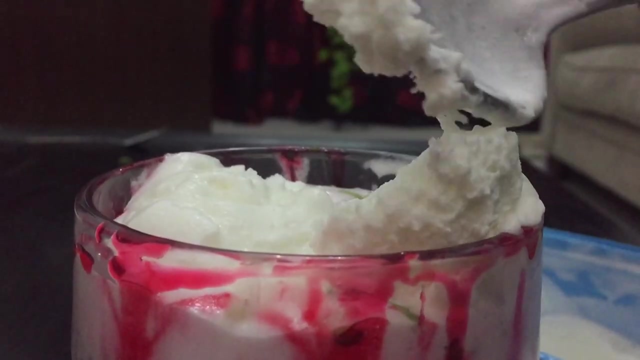 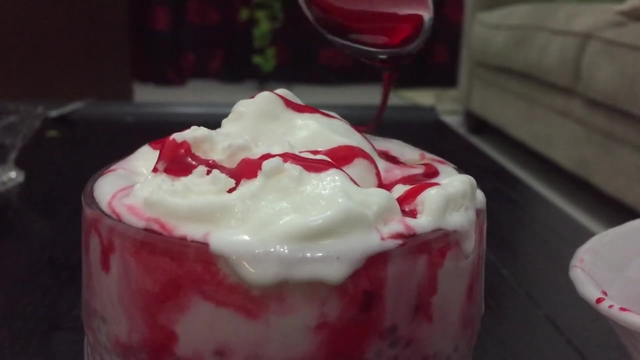 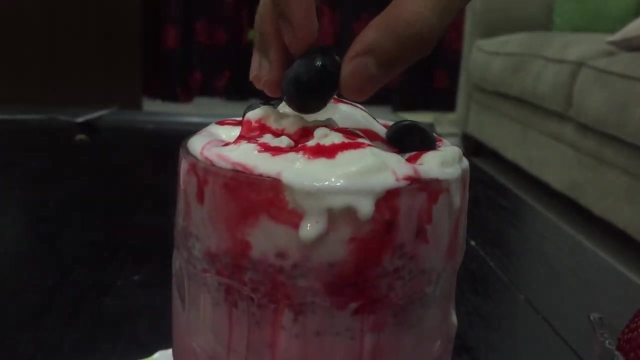 Now I am adding the walnuts. Now we are adding the milk. Now we are adding the walnuts. Now we are adding more ice cream. Now I am adding blueberries and strawberry. The blueberries are actually kind of sinking in right now. 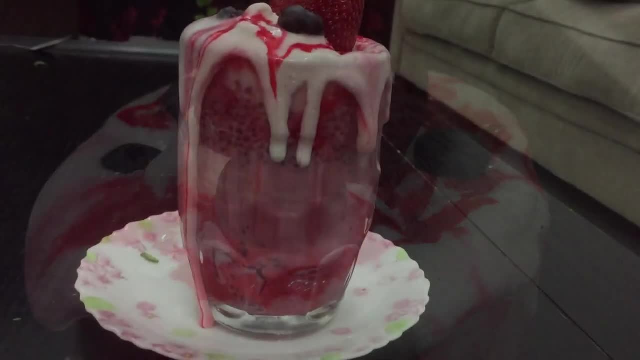 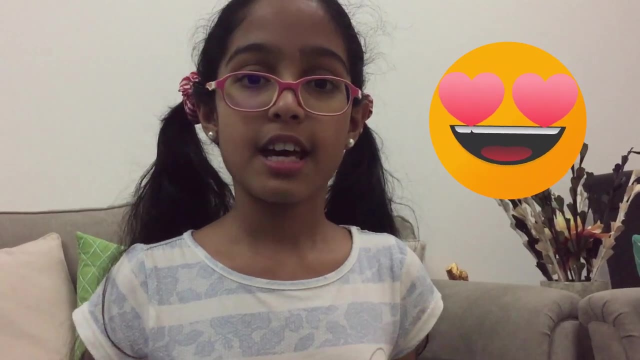 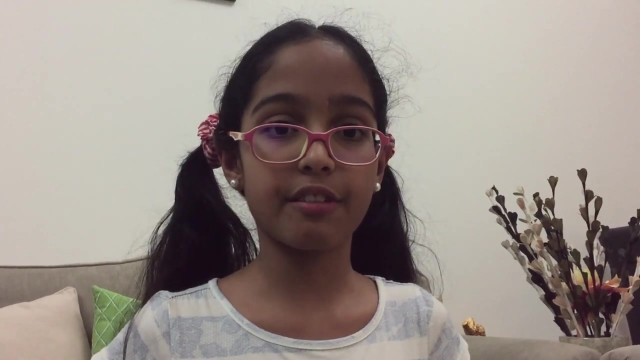 The blueberries are actually kind of sinking in right now. The blueberries are actually kind of sinking in right now. So, guys, we are done with all the recipes, and now we are going to be revealing all the end results of the recipes that we have done today. 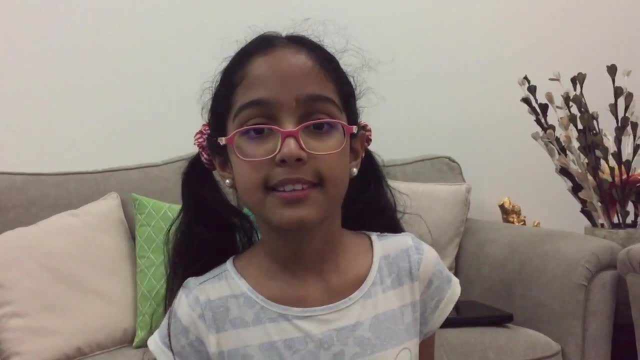 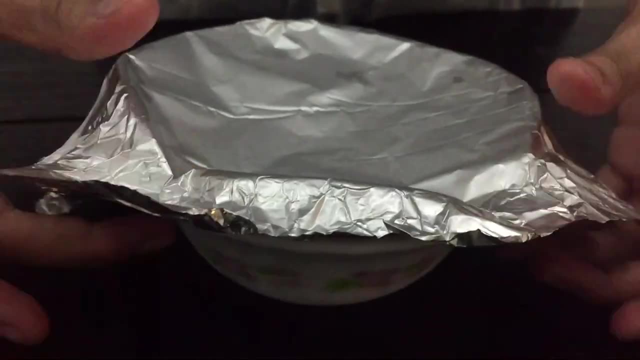 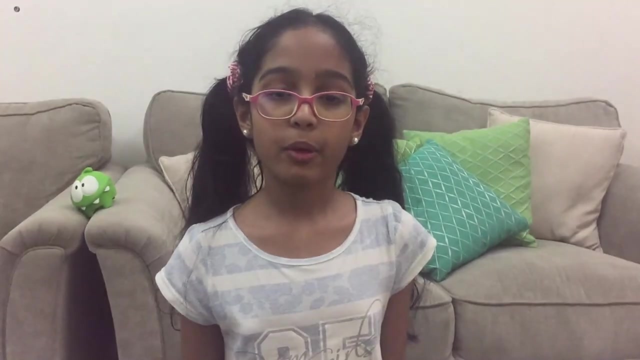 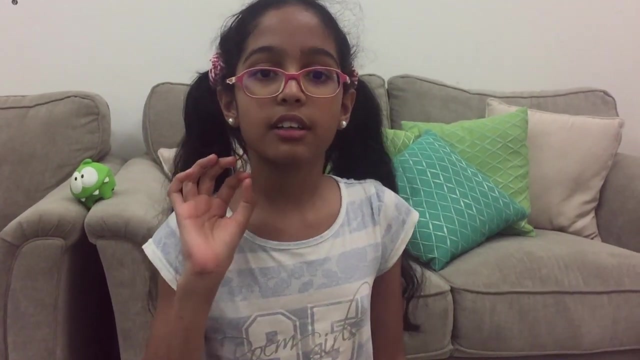 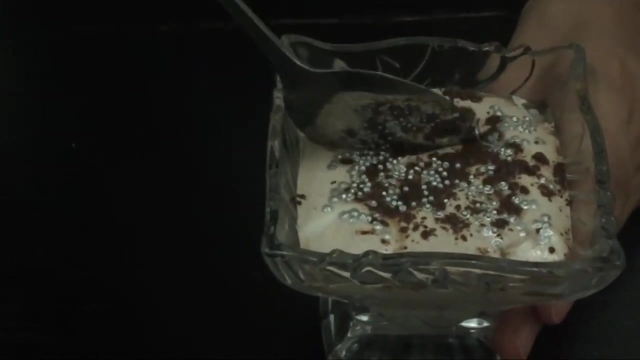 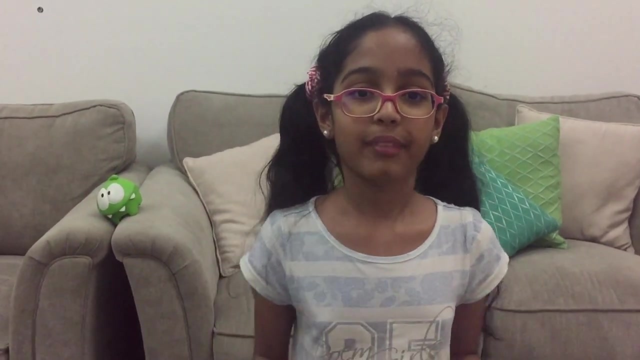 Starting with the chocolate mousse. Now, guys, I am going to do a taste test and I am going to describe every last bit of how all the recipes taste. First one is chocolate mousse. let's just cut into it. it tastes really good, it tastes. 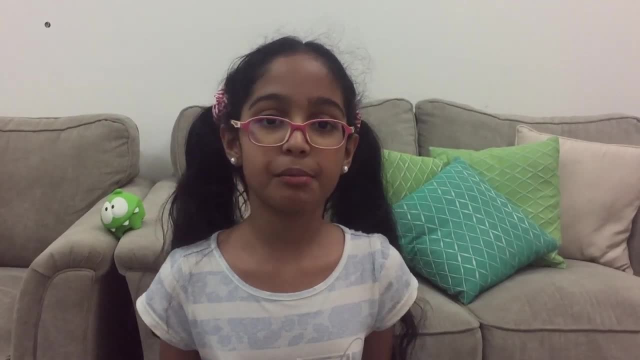 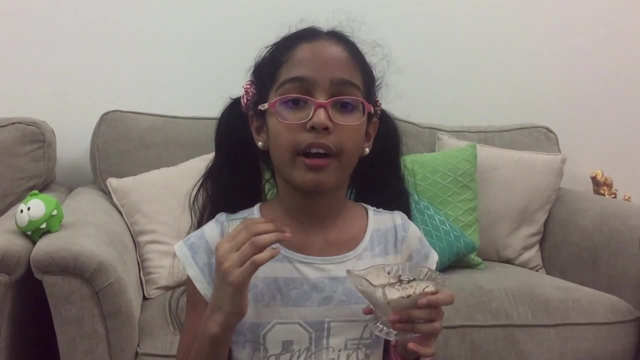 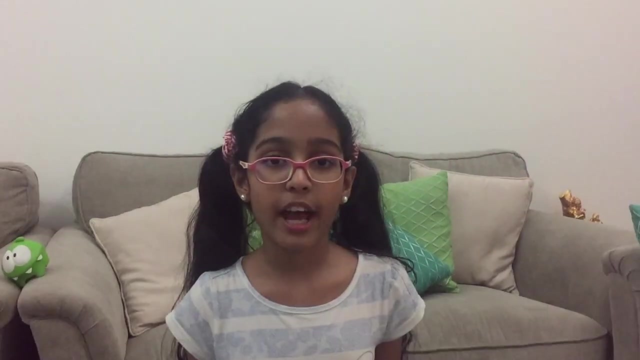 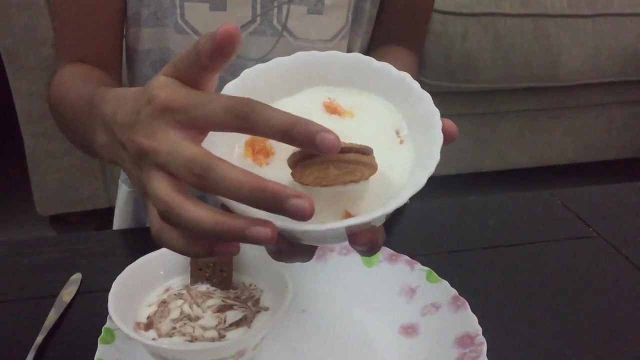 like chocolate, but a little bit lighter because of the cream. it is really delicious. it includes very few items and you guys must try it. Next is the biscuit ice cream cake. first we are going to be trying the orange flavoured one. as you can see, we have an orange biscuit, so it can actually look cool, and we have orange. 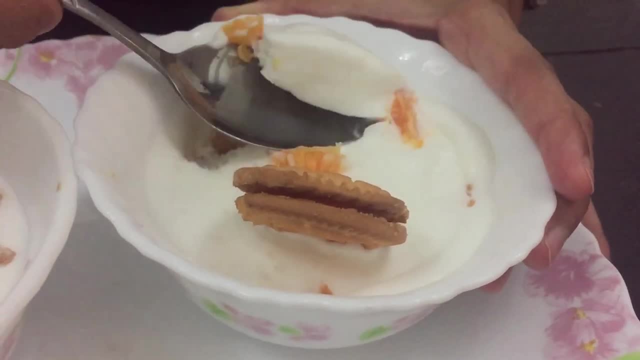 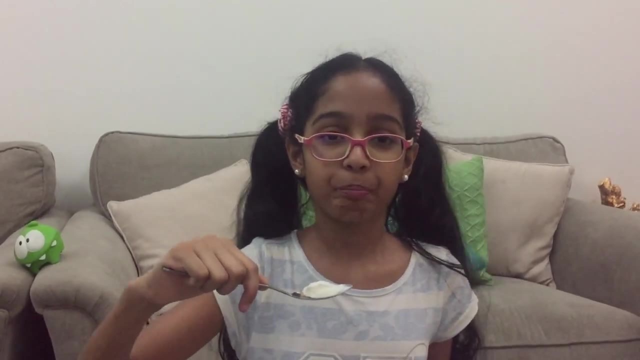 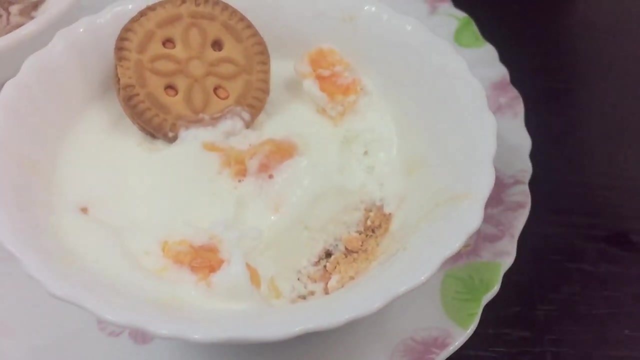 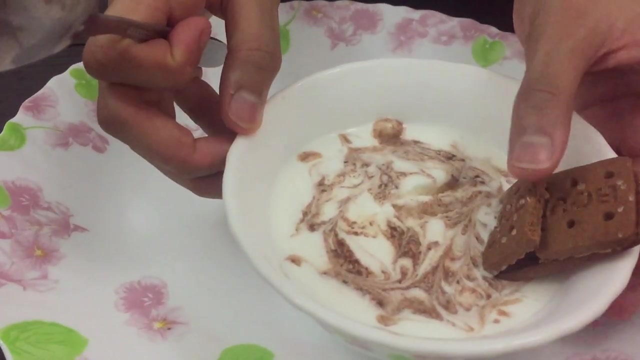 chunks. It's really good. we have added a little bit less biscuit, but you can see the layer here. you can add more biscuit if you want and do it in a bigger bowl if you want. Now we are going to be doing the chocolate one. as you can see here, you put a chocolate. 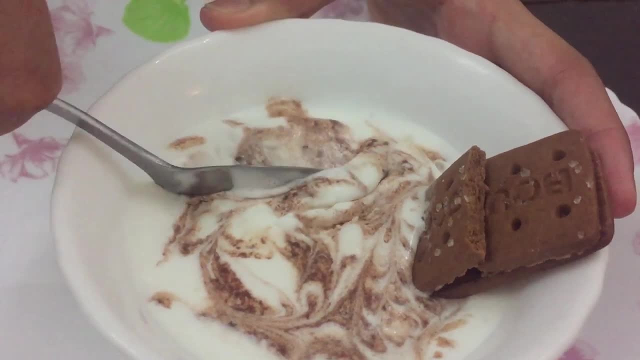 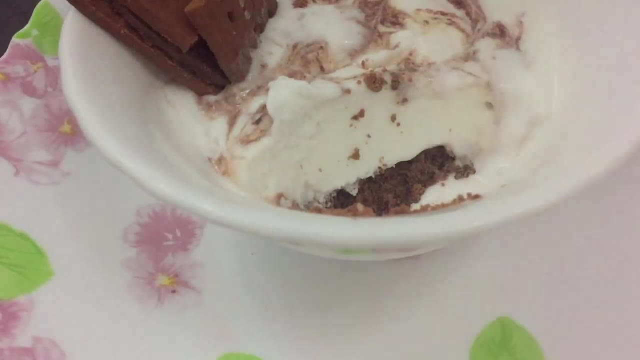 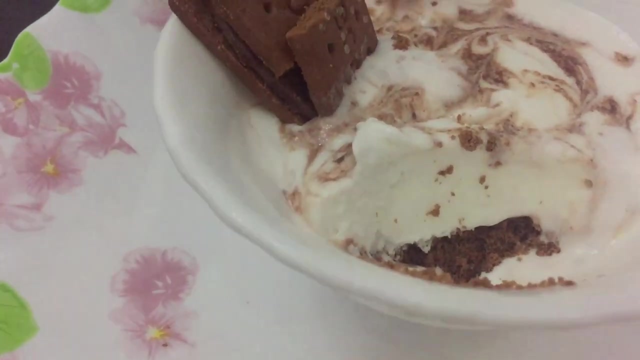 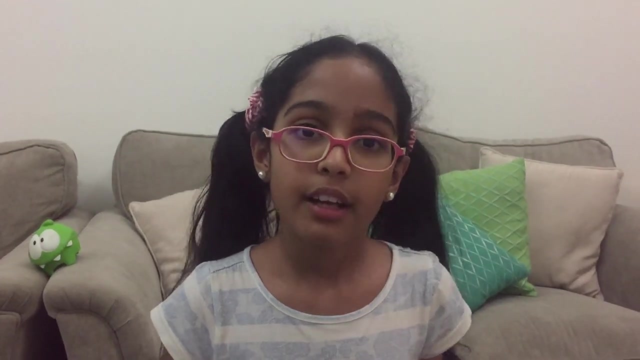 biscuit on top pour one. Now we put little bit more than the orange one, the biscuit. as you can see, the layer is little bit thicker here. This is a must try. it's so delicious even with plain vanilla ice cream. the biscuit's 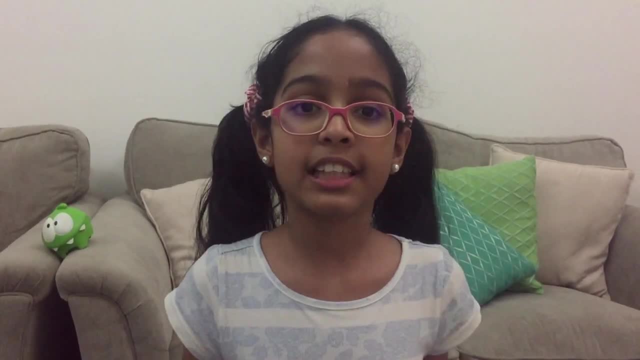 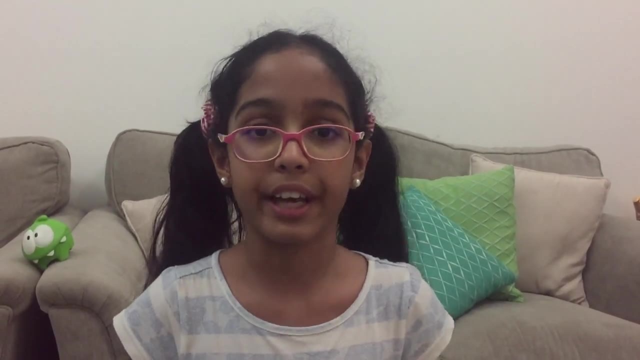 flavour makes it so that you are. it feels like you are actually eating a different flavoured ice cream, but with crunchiness. It's really good. It's really good, The crunchiness, it's so satisfying. The last dessert is the falooda. 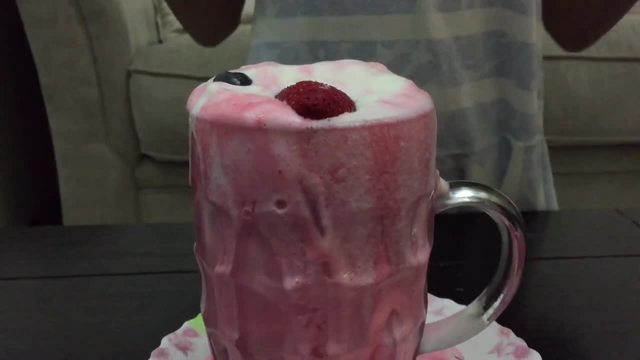 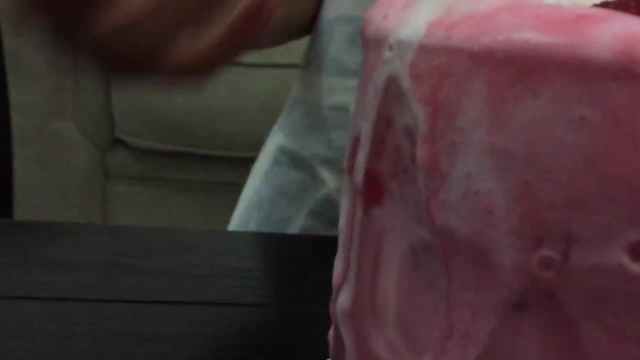 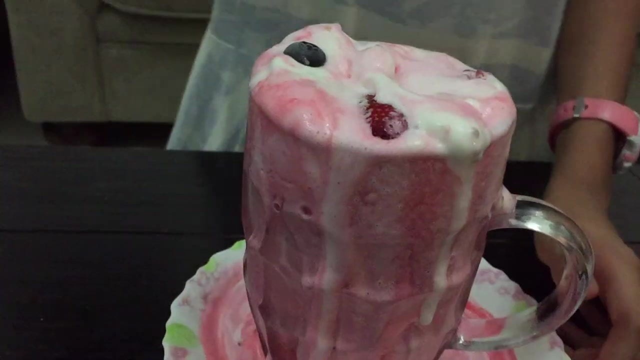 Look at this. I just don't want to eat it. I am afraid I will ruin it. I just want to keep it as a decoration. Just look at the layers, look at the drippiness, But I still have to eat it and then describe how it tastes. 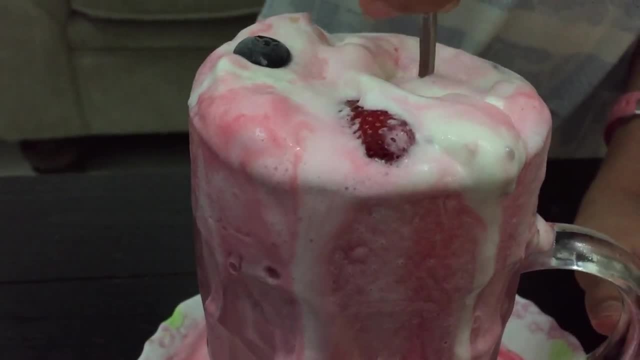 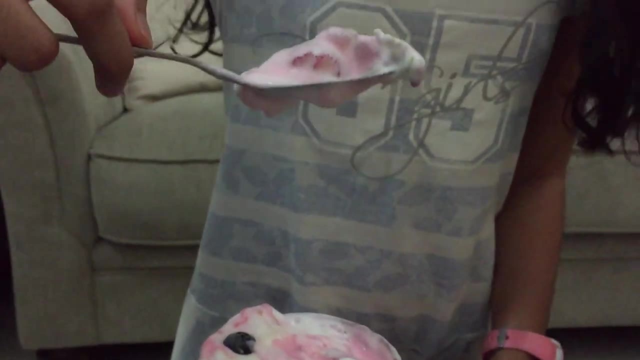 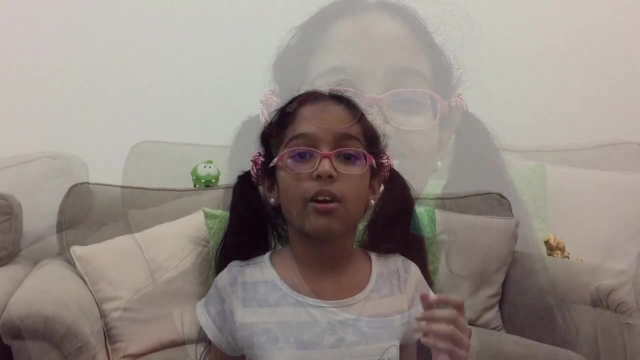 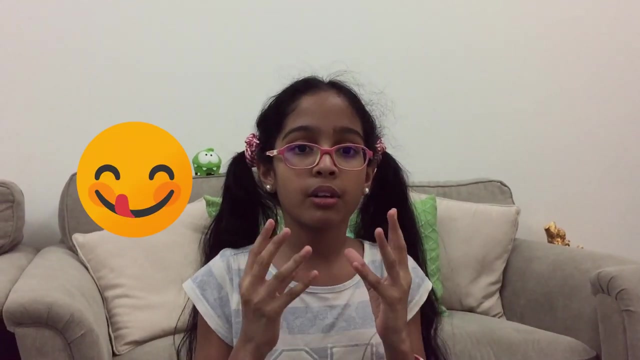 Here. you have to just dig down deep enough so you can get just enough and every every thing right. Guys, this is also a must try. it's really delicious Because of all the flavours that start bursting in your mouth. it feels so satisfying to just 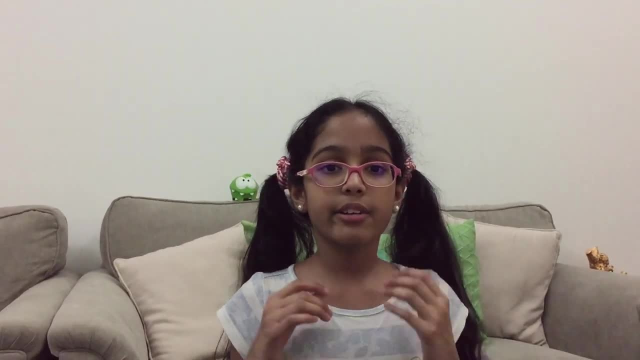 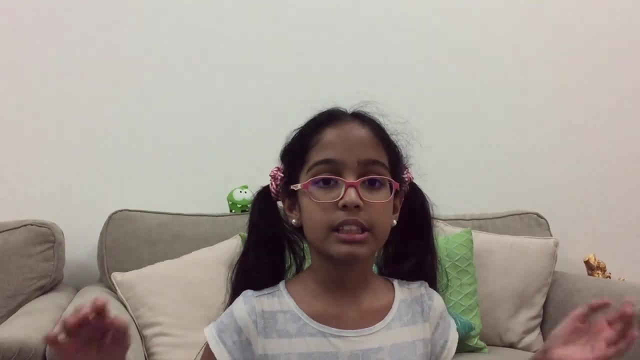 have it in your mouth, And it's also really nutritious because of all the nuts we are adding: the berries, the fruits, The milk, the sabza. This is so many things good about this that I can't explain myself, So that's why you also need to try this. 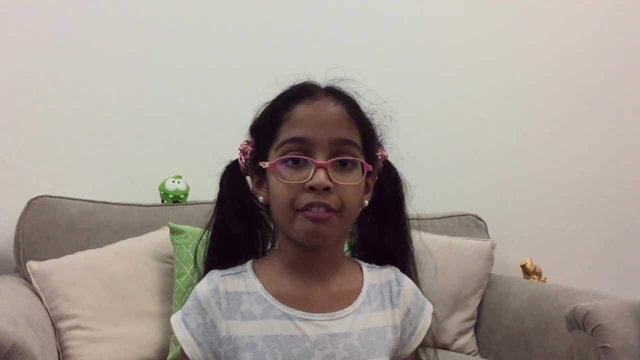 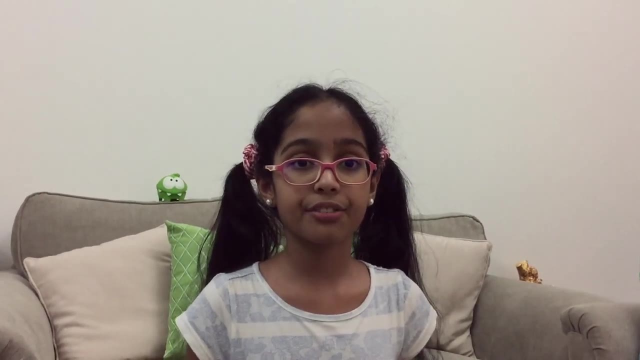 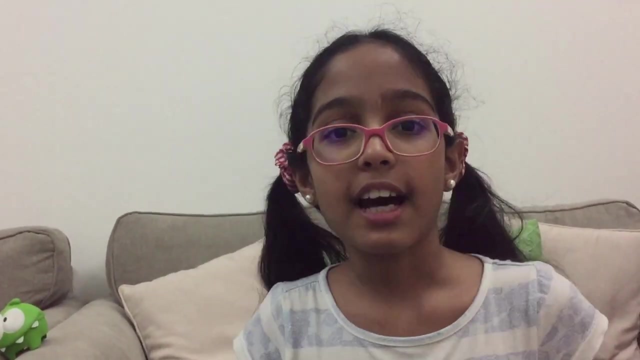 You can either eat it just directly after you made it, or you can freeze it for a little while. so all the ingredients, or some of the ingredients, can just freeze together. You can use any toppings you would like, Any fruits, any berries or any nuts.